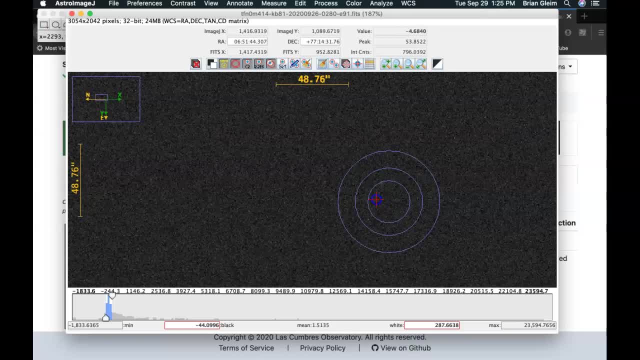 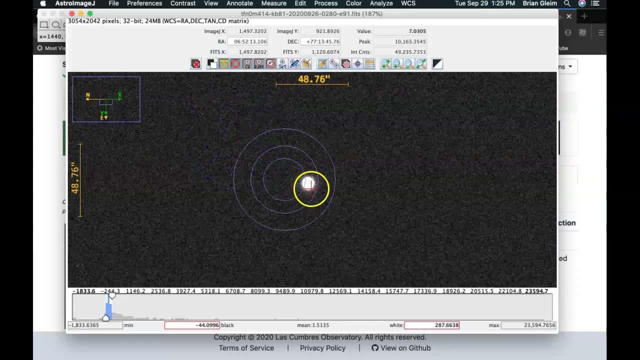 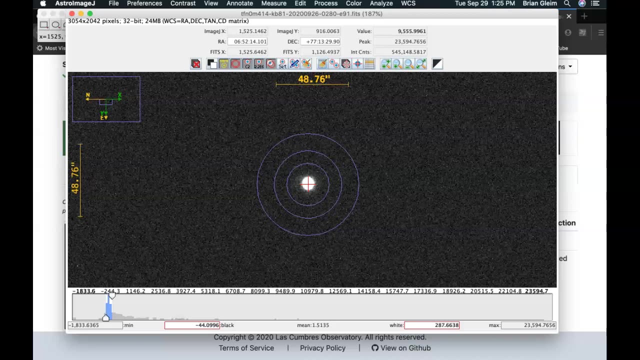 So that's your field of view, So you can move around and it'll move the purple box that shows you what your field of view is. So probably that's our target star. I say probably. We want to be sure, right? If you want to look at a particular star, double check okay. What are all these? 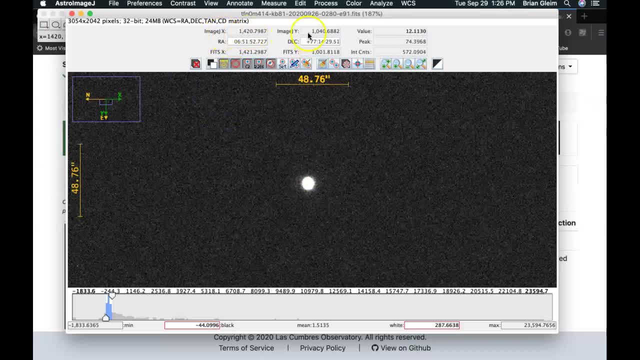 numbers up on the top here. So image J, X and Y. those are the X and Y coordinates for the pixel that your mouse is hovering over. So that's just telling you the coordinates on the image in X and Y coordinates. 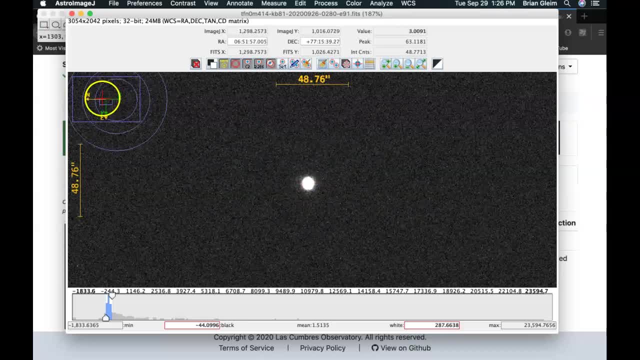 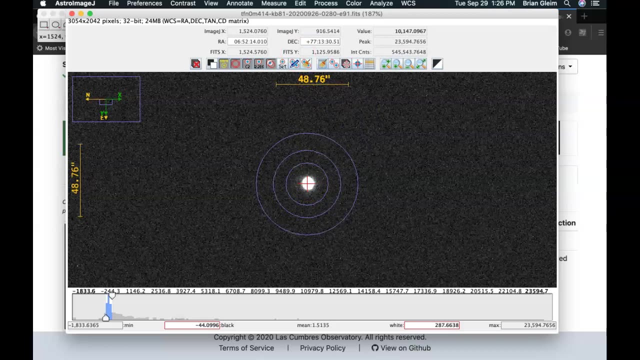 where again the green arrows here tell you: X increases to the right, Y increases going down. The more important part here is right ascension and declination. The other important thing about FITS images is that every FITS image has a text file appended to it, called a header. 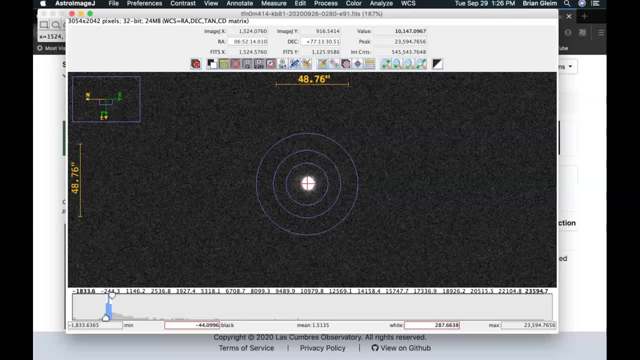 So when the telescope takes the image, the software on the telescope is automatically set up to glue this header onto the image And the header has lots of valuable information about the image. One of the things that the header has is the right ascension and declination coordinates where this image was taken. So the software here 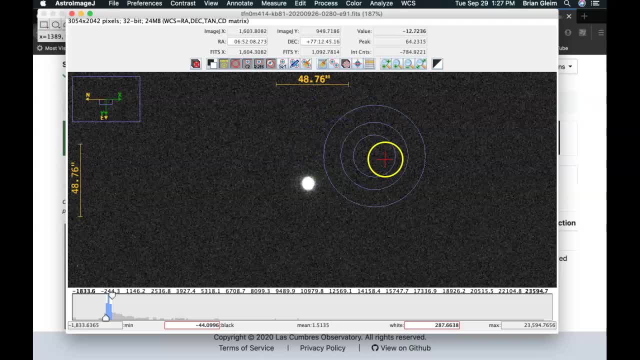 Astro Image J reads off the header and it says: okay, based on what the header is telling me, it can convert the X and Y coordinates in this picture into right ascension and declination coordinates on the celestial sphere. Here's how you read this right. This is a sort of a standard. 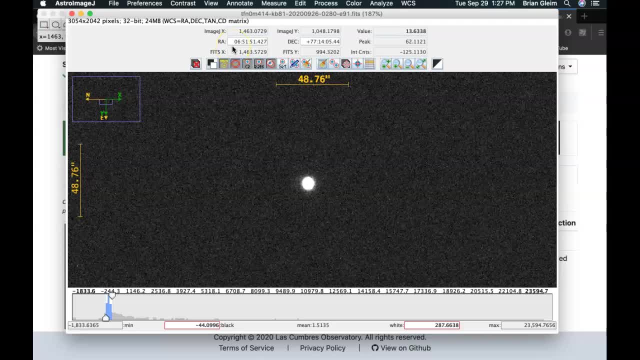 way to read or to notate right ascension and declination. So remember right ascension and is measured in hours, minutes and seconds. so those are broken up with the colons. so that's so wherever my mouse was a second ago, that is, that point is at six hours 51 minutes 51.6 seconds of right. 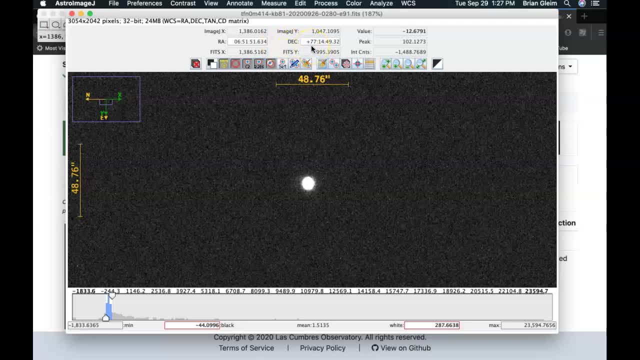 ascension and positive 77 degrees, 14 arc minutes and 49 arc seconds of declination. okay, so you want to go and say, oh, okay, that's my target star. all right, you can click on it if you want to. um, oh, i don't have it set up to do anything if i click on it, but okay, um. 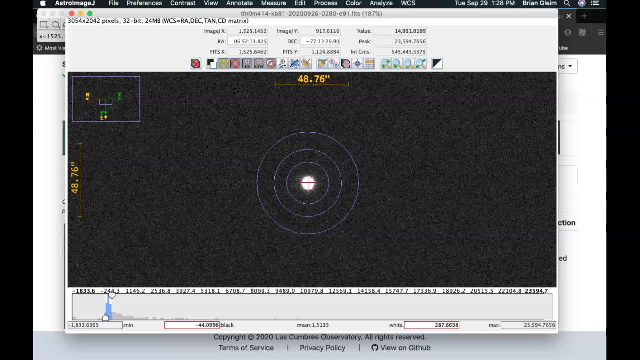 hover your mouse over that star and then double check: is this the correct right ascension and declination for my target star? it probably is. the pointing on these lco telescopes is pretty good, so i'm going to go ahead and do that, and i'm going to go ahead and do that, and i'm going to. 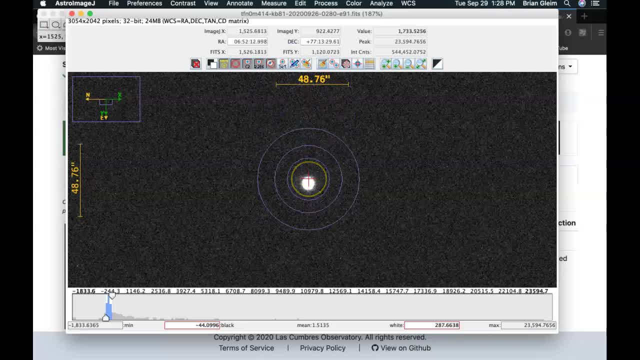 um, but you just want to be sure, is this the star i'm studying? it's at the right ra and deck. it must be the right star. okay, this is, this is the one i'm going to study. if it's not, then you need to sort of go hunting around and go: well, okay, which one of these stars is it? uh, oh, maybe, oh. 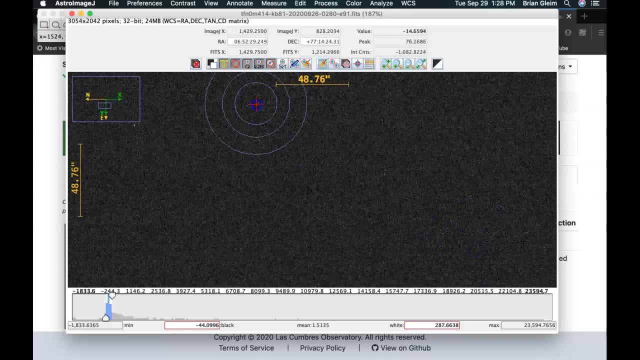 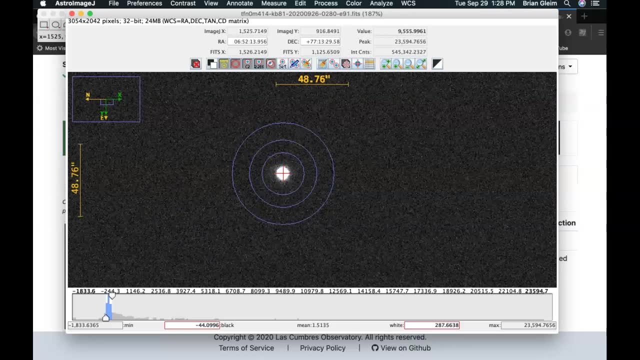 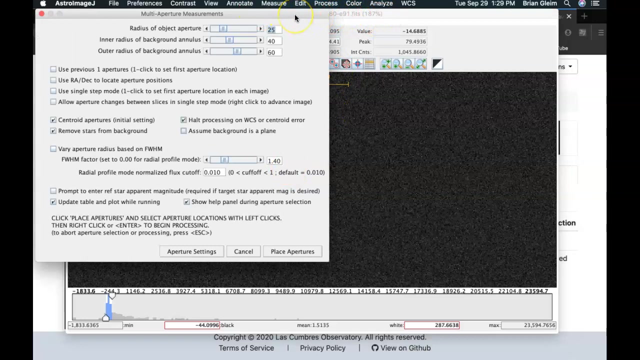 it's that one. oh, okay, there you go. all right. um, just a good sanity check. you don't want to spend hours studying the wrong star, right, um, okay, okay, um, to measure the brightness of the star, you need to, like we were talking about before your. uh, i'm gonna do here, we go, okay. so, um, multi-aperture photometry- okay, i'll explain. 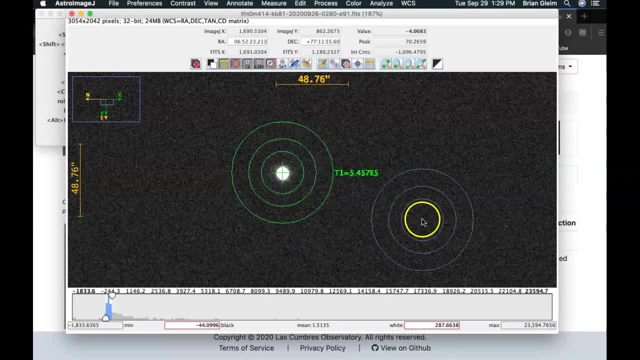 this here in a second, but i just want to like paint this on here to uh, to show, just to show the point. um, all right, we're going to draw three apertures, three circles around that star. all right, the, the software, is going to add up all of the light from inside the inner. 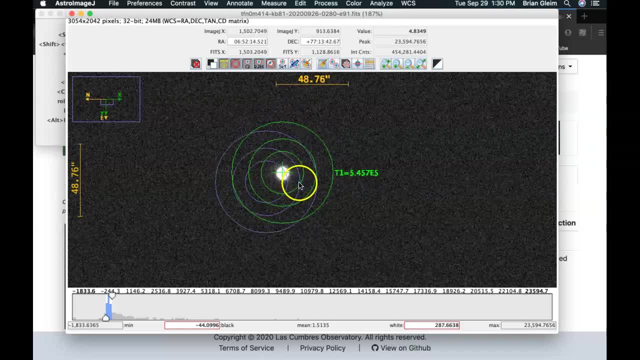 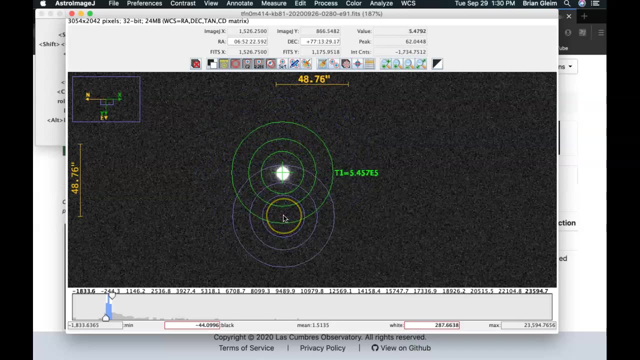 circle, and that's inside. this inner circle, should be the light from the star, but it's also going to be the extra light from the sky. then, in between the second and third circles, the software is going to sample how bright the sky is and then it's going to add up all of the light from the 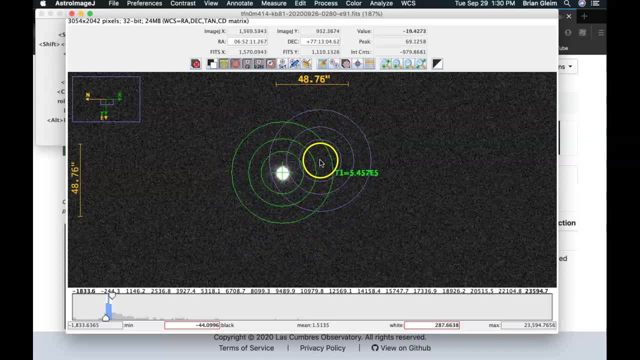 sky and it's going to subtract off. it's going to, by measuring how bright the sky is. it's going to subtract the light from the sky in this inner circle, so that what it spits out to us is just the light from the star right. it's going to take the light from the sky plus the star, subtract off. 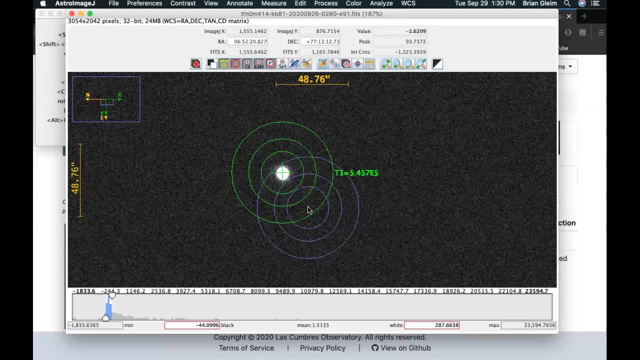 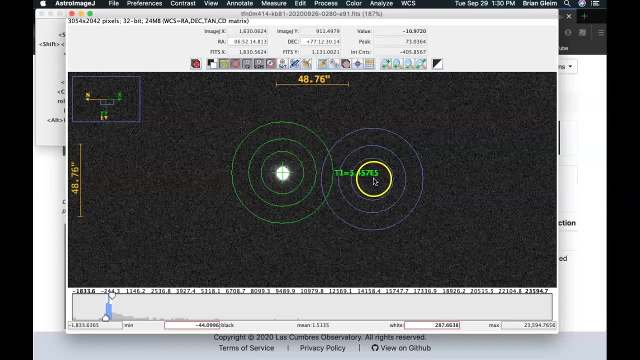 the light from the sky and it'll give us the brightness just of the star. now, that's probably what this number is right here. but so that that number right there, t1, t1 meaning target one, five point four, seven times ten to the fifth power, that's probably the. 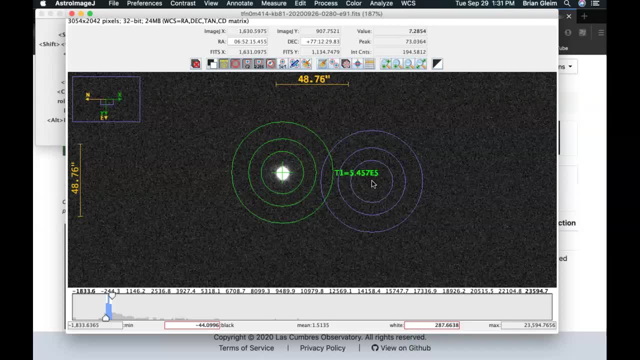 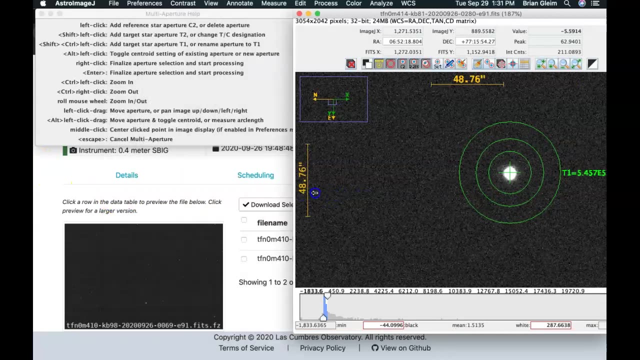 brightness inside there. but I want to be sure. I want to be sure, but also I want to know what the signal-to-noise ratio is. okay, how do we do that? okay, I'm gonna shrink this down for a second to do the photometry and to have it read off the answers to us. 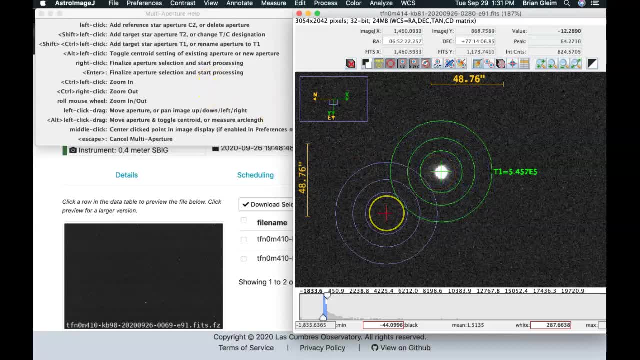 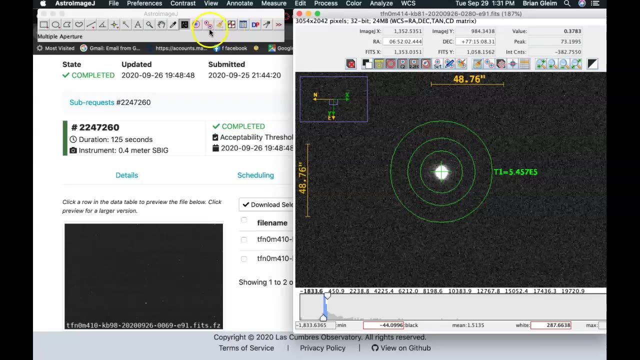 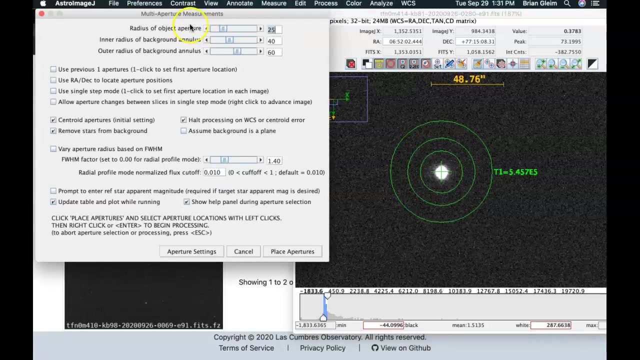 read off the measurements to us all. right, I I am going to go back here to the main menu. go to the, the two circles here that are called the aperture photo. sorry, multiple aperture. click on that. it's gonna give you the a bunch of settings. I, as of right now, I think these settings are fine. 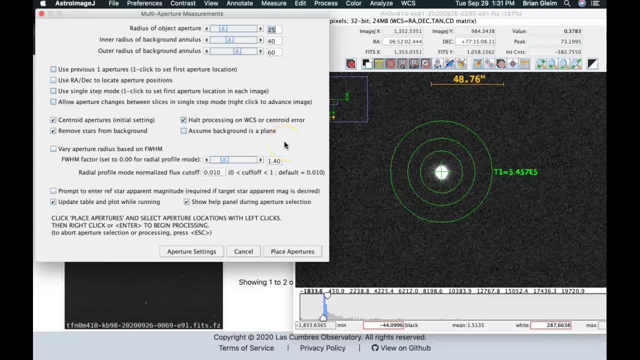 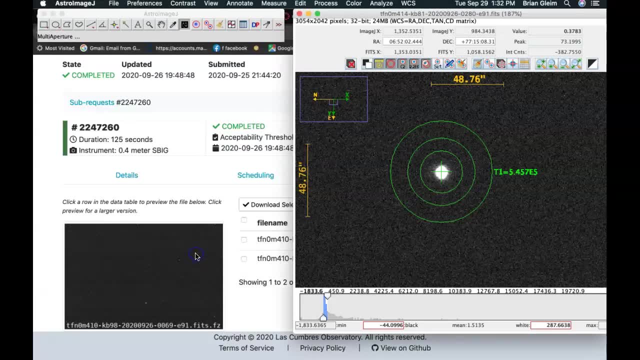 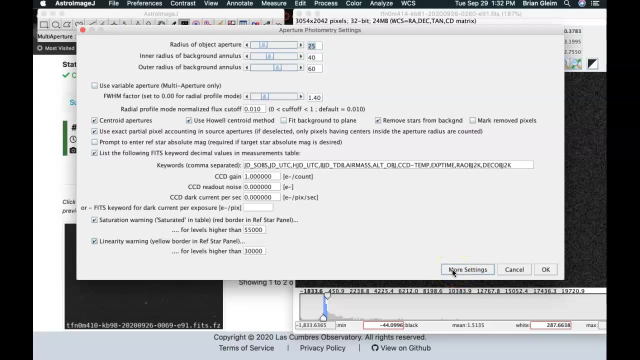 we may need to tweak these later, but these are the default settings that I'm seeing and it seems okay to me. just leave these as is for right now, go to aperture settings and it's gonna give us, I think, the same thing. so just leave these as is for now, click more settings and now it's gonna. 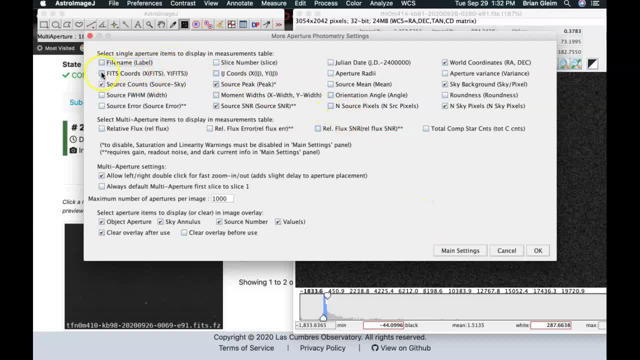 say: all right, what all? what all measurements do we want to take? each of these click boxes is a measurement that we could have the software spit out for us, the file name I. I unclick this. yours is gonna look different because I was playing around with this earlier, but do I? 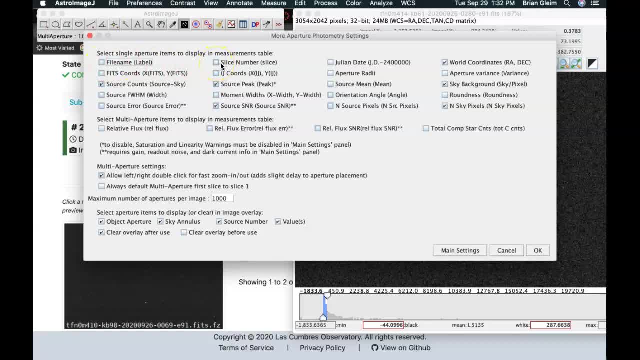 need the file name. no, I don't need the file name. uh slice number net- Julian date. Julian date is an astra astronomical way of measuring time and date. you don't need that. click that off. world coordinates in right ascension and declination. I want that the X and Y coordinates. 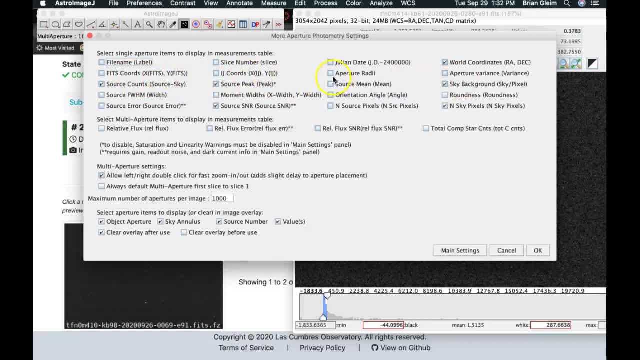 and no. X and Y coordinates, don't care, aperture radius, not that important. the source counts this. this is what I want, right? I want to know what are the counts from the source, the source in this case being the star. what is a count? a count is an electron right? how many electrons did the 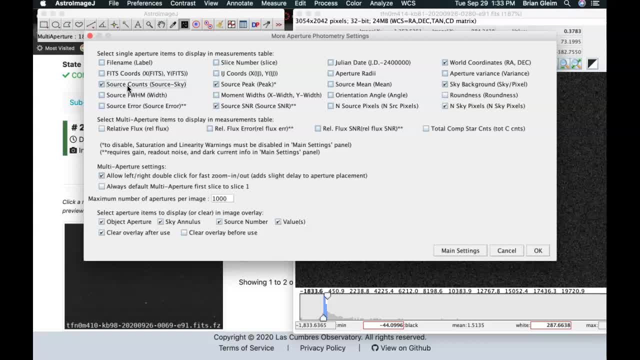 light from that star generate on my CCD. so the quote-unquote counts are what we're measuring, because the counts are proportional to the flux, right. so that's, that's our main answer here. the source Peak: eh fine, um sky background. I want to know how bright the sky is. 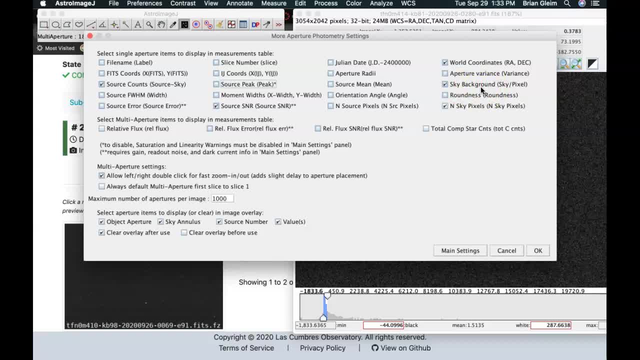 because that'll give us a sense of, um, how noisy our information is. uh, I unclicked all of these, but I want to know the source. snr, snr- is the signal to noise ratio right? the signal is the light from the star, the noise is the light from the sky and all the other error sources. so by taking 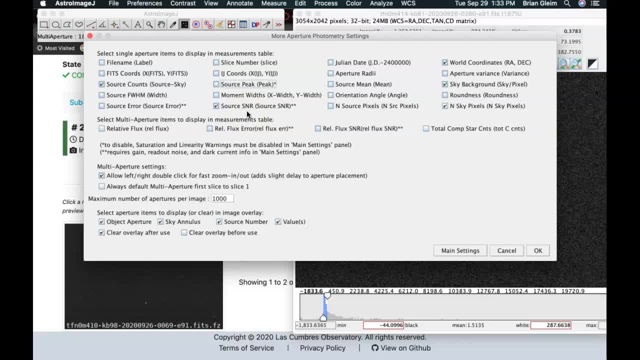 the signal to noise you take. you take how much light or how many electrons did we get from the star? how many electrons were generated by the noise? when you divide them, that gives you a measurement of the error, of how good your data is, how reliable it is. the higher the signal to noise ratio, the 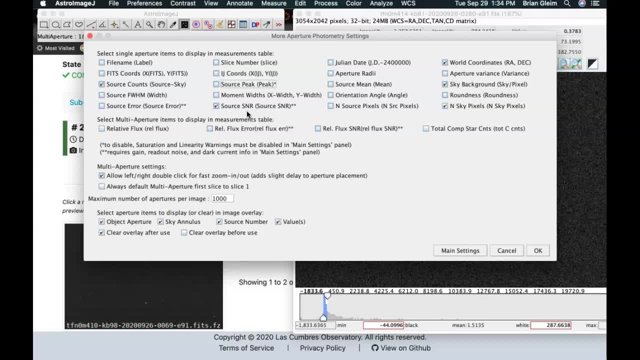 cleaner our signal is, the more reliable our measurements are. so those are the three main things that I want: source counts, sky background source, signal to noise ratio. those are the three things we want I. I could pretty much unclick all of these- oh, and the RA and deck. 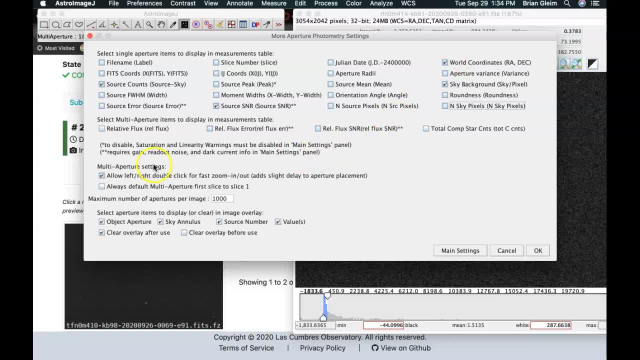 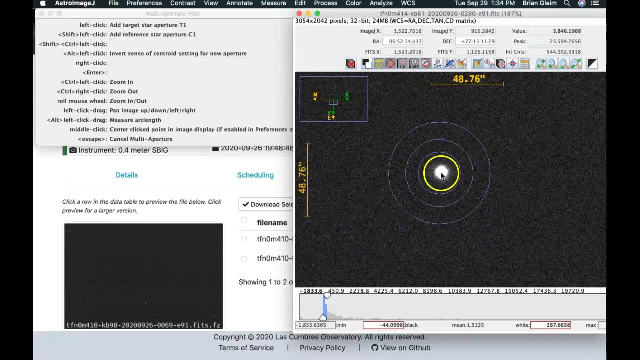 is good, just to be safe. um, I'm gonna unclick. I'm gonna leave the rest of these as they are because I haven't played with those yet, so I'm gonna leave those as is. I click. OK, all right. then I say place apertures. all right, now I'm ready to do what I just did. I'm going to click on this right. if I were. 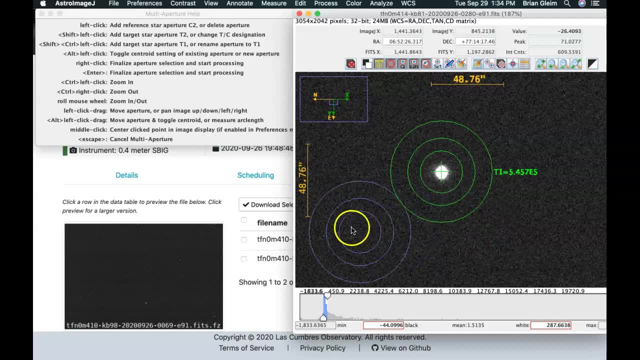 doing more than one star, then I could click on multiple star. then I could click on multiple star, multiple stars and click. you know measure multiple stars at once. but I just want to do this one, So I left. click on my star. it places my apertures Once I'm done and I'm ready for my 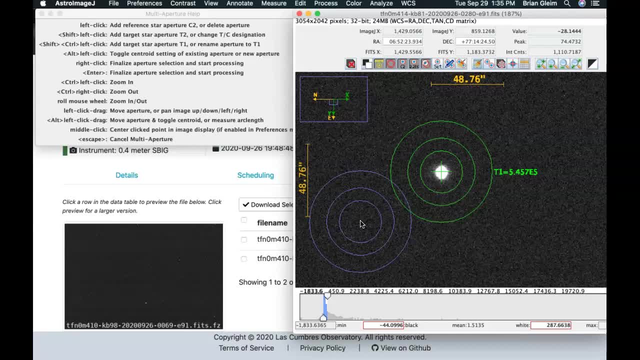 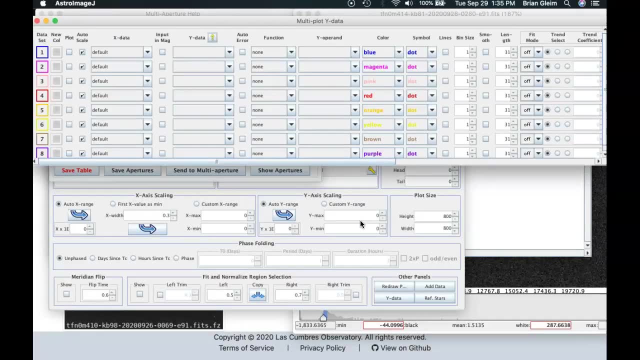 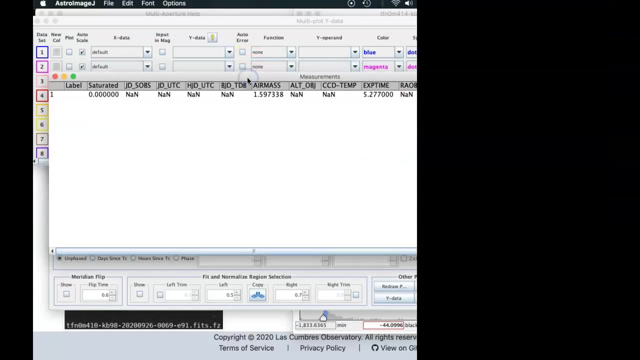 brightness to be processed. I right click on the image and then the program just starts spitting out lots and lots of windows. I don't know how to turn these off yet, but you know, the one important thing that we need is the measurements window right here. This is our answer, Oh, and 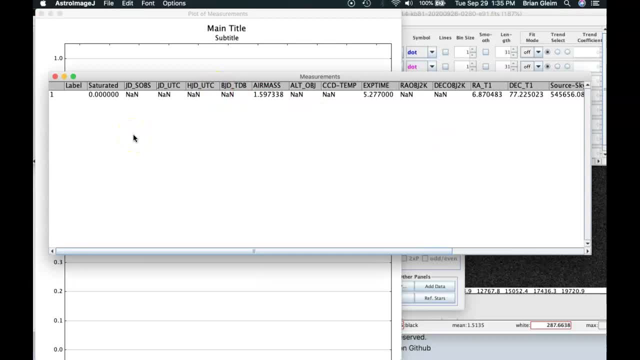 that thing. Okay, We don't need that. So this is all of the measurements for my star. So here's my source, my source: brightness right, Half a million counts. Cool. My signal to noise ratio: 736.. So the? 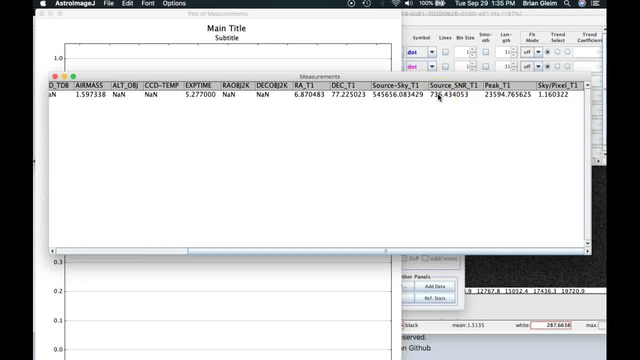 star was 736 times brighter than the light from the sky and all the sources of noise, So that's a good ratio. That's a very, very good ratio. The sky per pixel is 1.1.. That's pretty nice, right. Basically, what that means is: 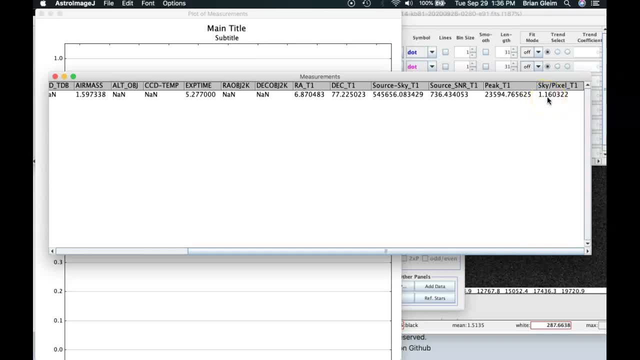 that every pixel of the sky is only generating one count. That's a nice quiet background. Ideally, if we could clean up the sky perfectly, it would be zero. but you know, one compared to half a million, one might as well be equal to zero. So that's nice. That's one of the reasons why our 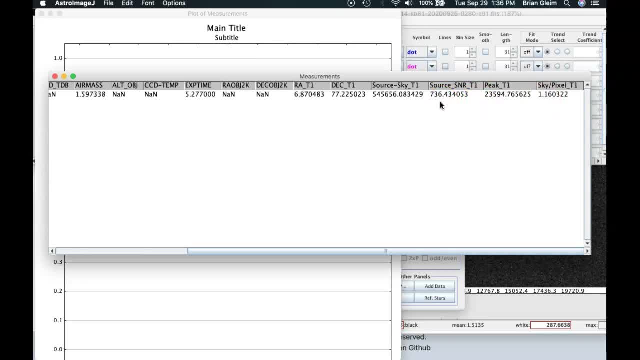 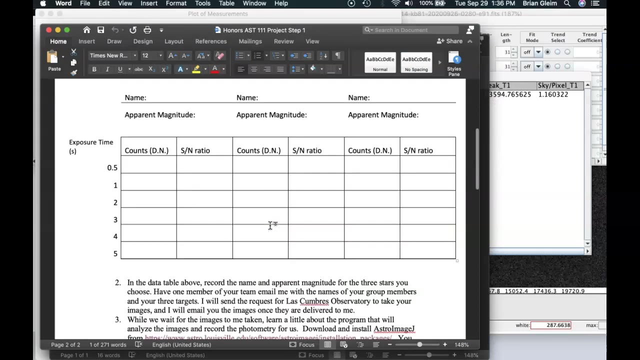 signal to noise ratio is so good, It's because the source is so much brighter than our reduced sky. Okay, So, on the instruction sheet that I gave you last week, I want you for for each right, For your, your bright star, your. 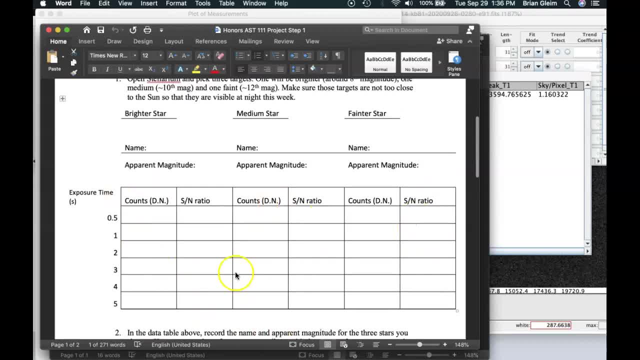 medium star and your faint star. right For the bright star, the medium star and the faint star. I want you to give me the counts and you don't really need DN. I, DN is one of the ways of measuring counts in a different piece of software that I decided to not have you. 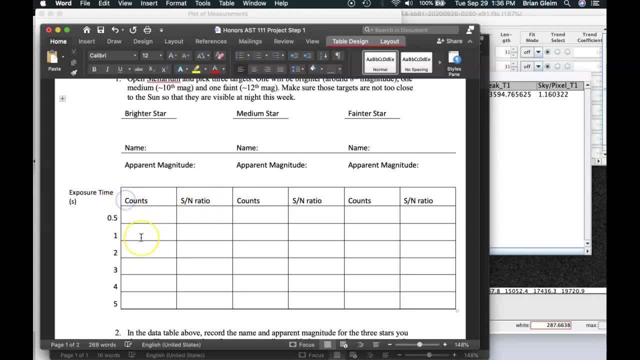 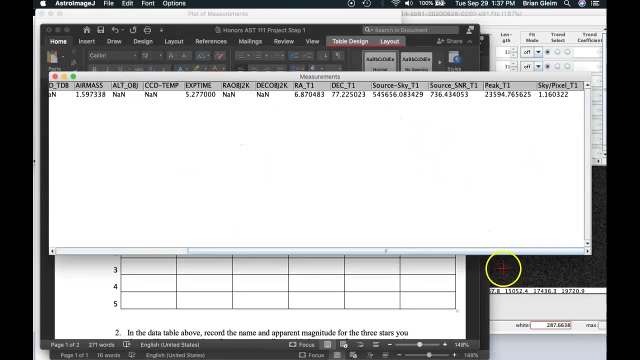 guys do, So we can get rid of the DN. I'll just say source counts, record for each exposure, the number of source counts and the signal to noise ratio. Those are the three answers we need for each image. Okay, How will you know which image right Is this? 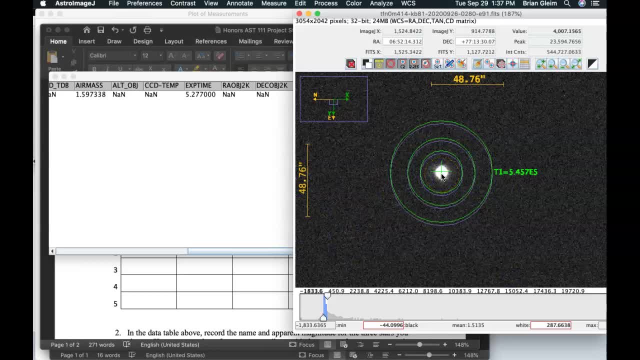 image of the bright star, the medium star, the faint star and what's the exposure time. that can be read right off of the header. So if you go up here to this, this button right here, if you leave your mouse it'll say display fits header. You click on that And this is the big text file. 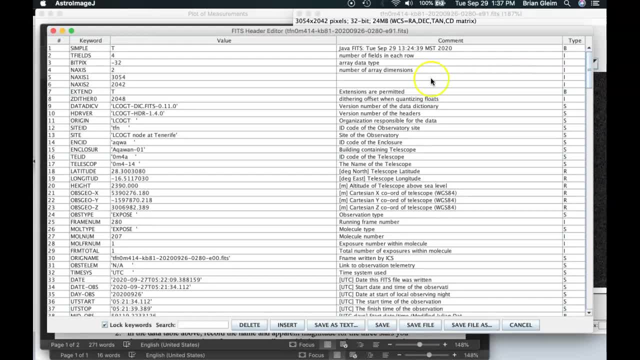 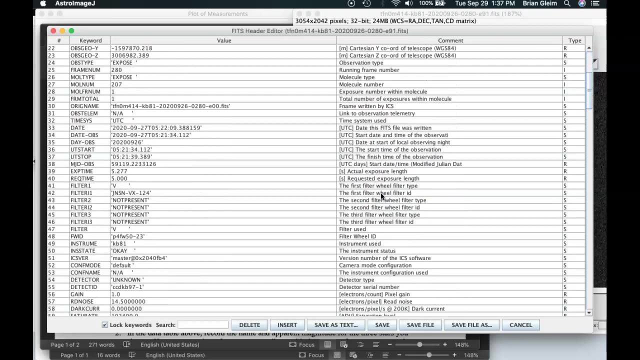 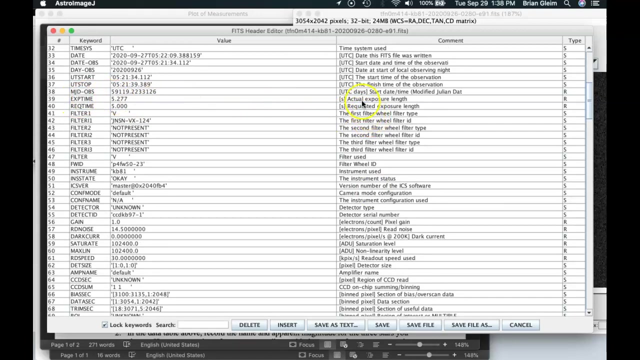 This is the big header that gets appended to each image. All right, Lots of stuff. It's like: here's the keyword, Here's the value, Uh, the. the comment column basically explains what each of these rows is. So what you want to know is column ah, column 39,. column 39 is the actual exposure. 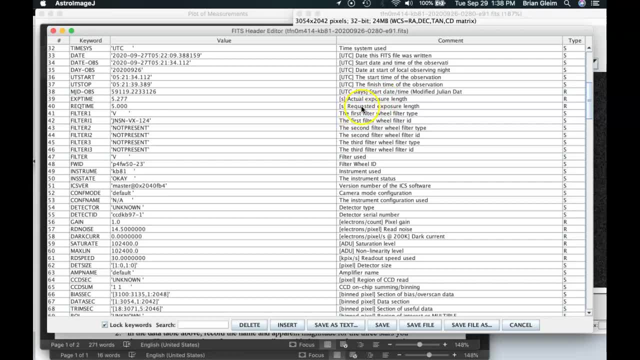 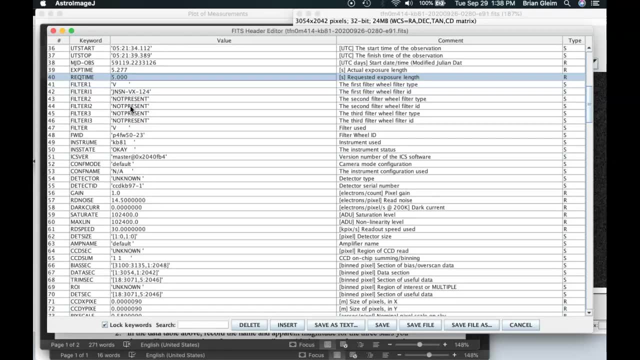 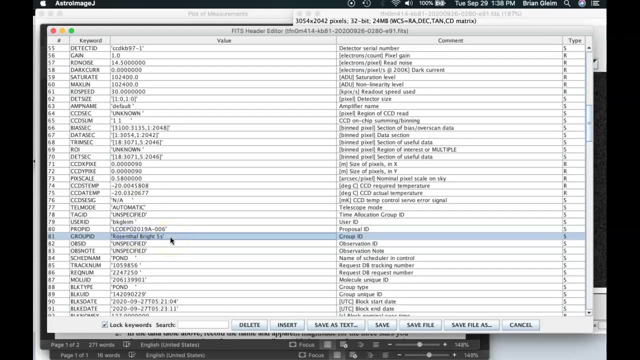 length, or you could go to column 40,, which is the requested exposure length in seconds. So this is the image that I requested be taken for five seconds And, ah, column 81,, that's, that was the name of my request. So, Rosenthal, bright number, five seconds. 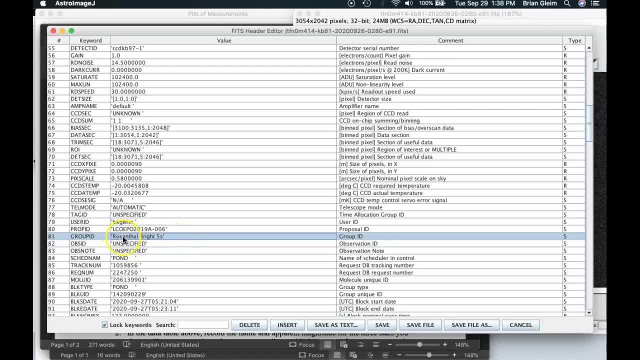 So that can help you out. right. This is for for for Genevieve and Andrea's group. your bright star, your five second exposure. So I sort of did this out of order. You could do this first, right. Open an image. open the image. open the header. figure out which star. 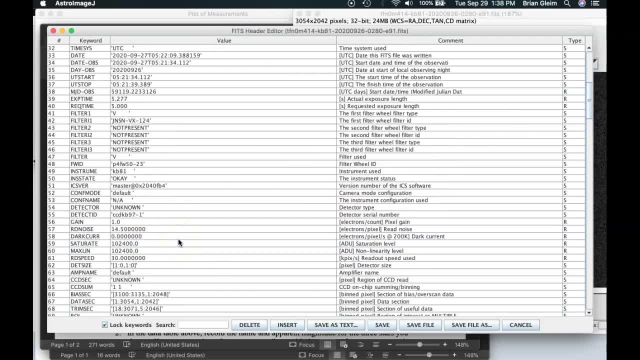 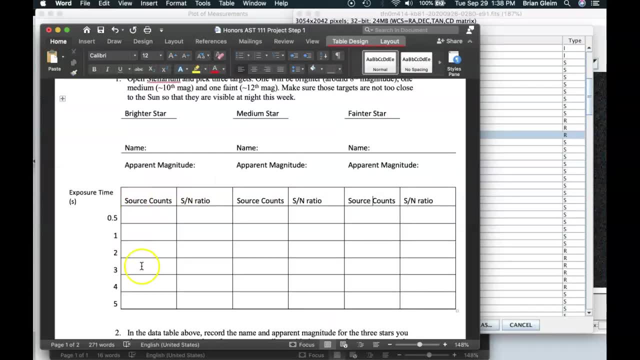 this is, This is your bright star, your five second exposure. Um, make sure that it's your five second exposure. Yup, It sure is Great. Now you know where you know. now you know. okay, so this is the bright star: five seconds. Okay, I'm going to write this in here. So then, 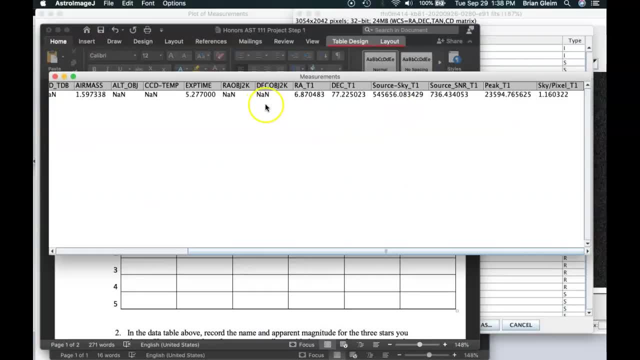 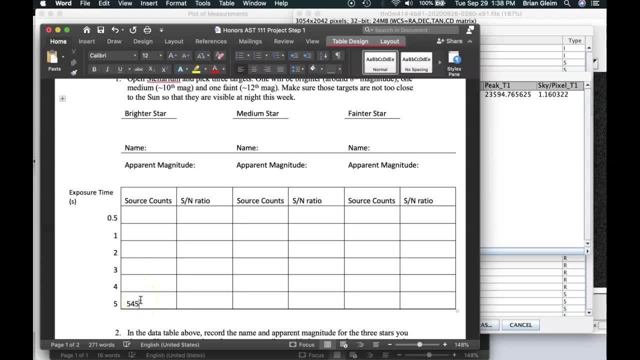 for this star, the bright star, for five seconds. uh, 5,, 4,, 5,, 6,, 5, 6 is your source counts, So 5, 4,, 5,, 6,, 5,, 6.. And your signal to noise ratio is 736.. Great, All right Onto the next image. right, You're done with this image. Go to the next image. You're done with this image. Go to the next image. Right, You're done with this image. Go to the next image. Go to the next image. Go to the next image. 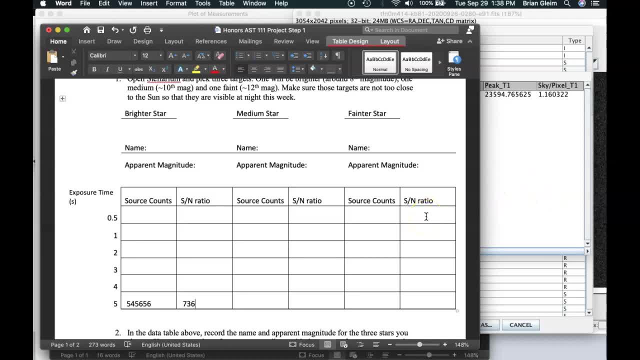 with this image, go do the next one. That's how you're going to fill out this table.